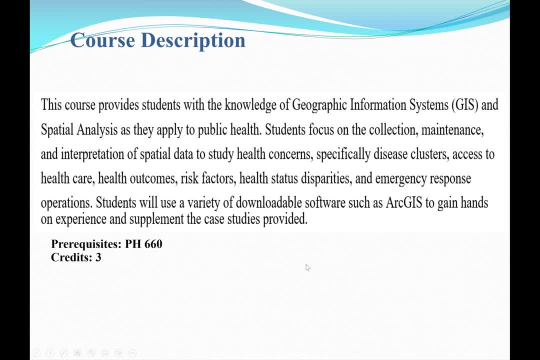 from GIS. Also, students will focus on the collection, maintenance, also interpretation of spatial data. A spatial data is a data that is related to a location, a geographical location, And also we are going to focus on a disease cross-test, access to health care risk factors. 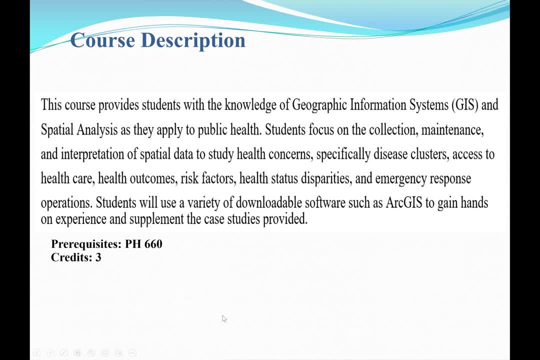 emergency response operations. Also, we're going to have a hands-on exercise and tutorial in this course. So we're going to have a hands-on exercise and tutorial in this course. So we're also going to have a hands-on exercise and tutorial in this course. So we're going to have 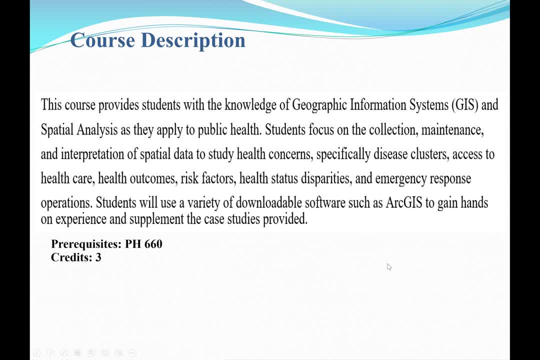 a hands-on exercise and tutorial in this course. So we're going to have a hands-on exercise and tutorial in this course using the ArcGIS or the QGIS. These are the two GIS software applications that can be used to again manipulate, manage and also interpret a data set. 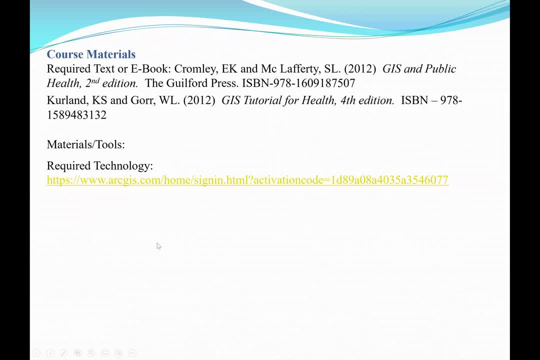 The prerequest for this course is the PH 660,, which is the Principles of Bowel Statistics, And the course materials is GIS and Public Health, Second Edition. And also we have a GIS tutorial textbook, And this textbook focuses on using the ArcGIS software. 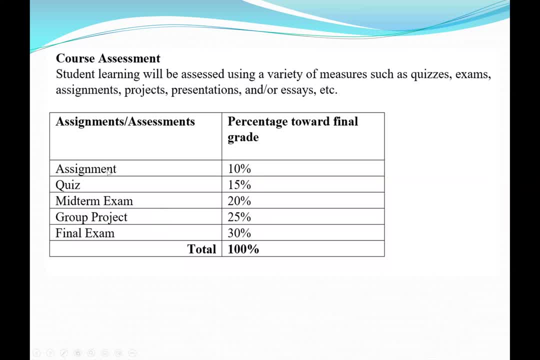 The course assessment. we are going to have bi-weekly assignments, which will be 10% of our final grade. We're also going to have three quizzes, which is 15% of our final grade. We're going to have one midterm exam- 20%- and also one final exam- 30%. 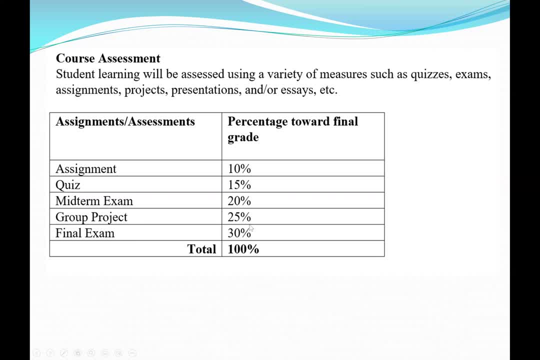 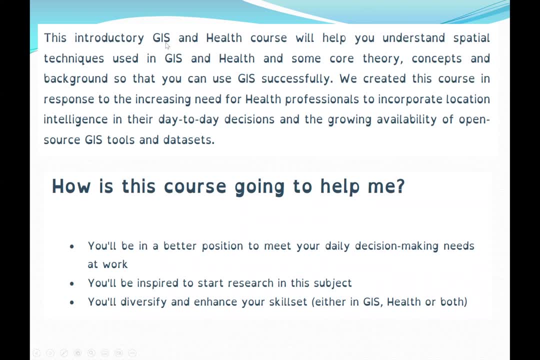 Then we're also going to have a group project, which is 25% of our final grade. So this is an introductory GIS course related to, again, health. So this course again will focus on using the GIS techniques and we are prior to mostly epidemiological data sets. 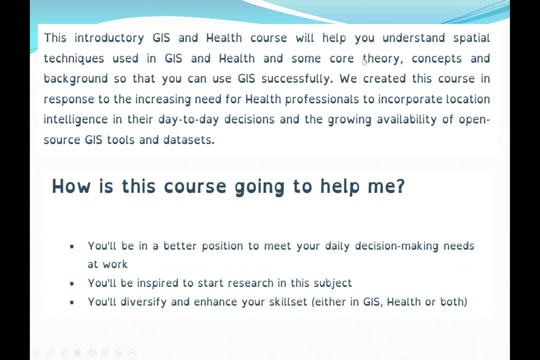 So, again, GIS and healthcare course will help you understand the data set. We're also going to have a course on spatial techniques using GIS and also health and some core theory concepts and background so that we can use GIS successfully. So how this course is going to help us, This course, again, will surely put us in a better position to meet our daily decision-making needs at work. 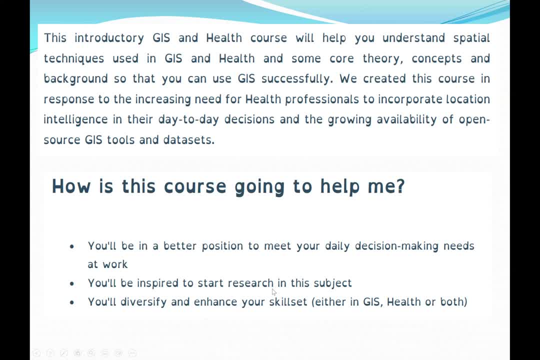 Also, it will inspire us to start a career in the field of health. We're also going to have a course on general health research in this subject. That's research in GIS related to, again, epidemiological data set or public health in general. 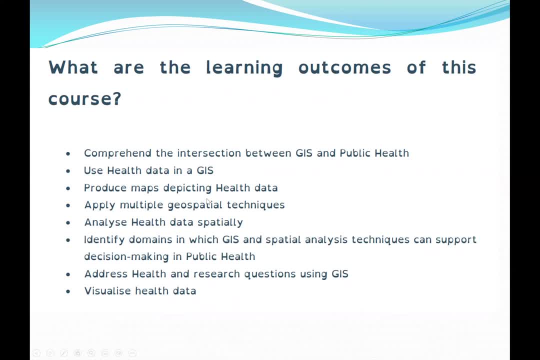 We're also going to learn some techniques on how to use the GIS software and apply it on public health data. So this is the course outcome: We're going to use the health data in GIS. Also, we're going to learn how to comprehend and intersect the data set. 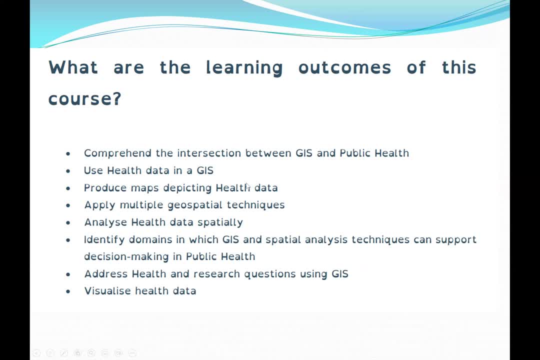 Then we're going to go through a summary with the performance, Then we're going to see if the piece of data is good or not. intersections between GIS and public health. We are going to learn how to produce maps showing health data and also how to apply multiple geospatial techniques. 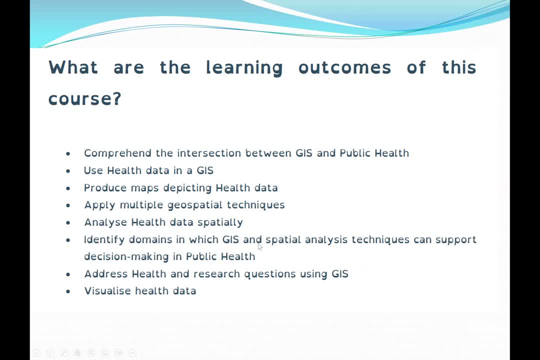 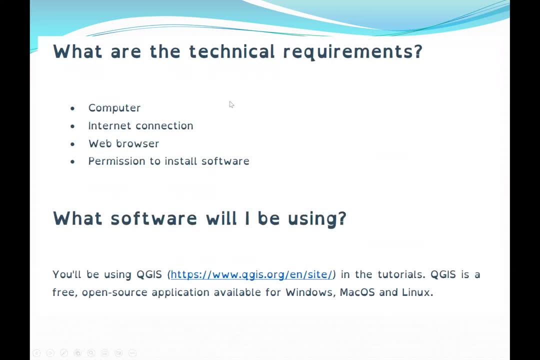 We're also going to analyze the healthcare data spatially and also how to visualize health data. So in this course we need a computer. since we are taking this course online, a laptop or a notebook is fine, or desktop computer. We need internet connection because again GIS software we are going to use and also this course will be online. 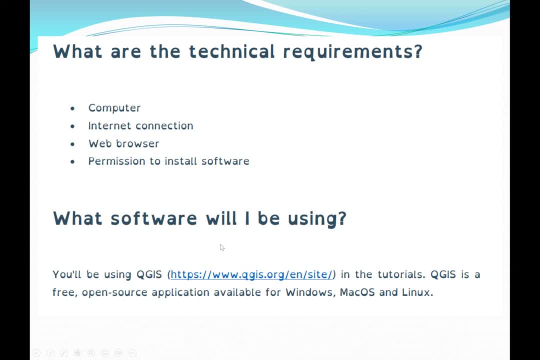 So the software we are going to use is the ArcGIS, which we have to get from the school, but we're also going to use QGIS a lot because this is an open source system and also is free. We can download it online for free. 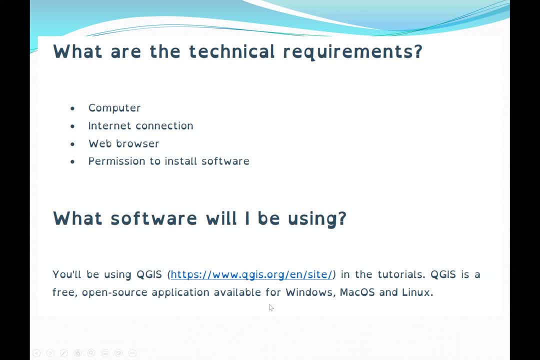 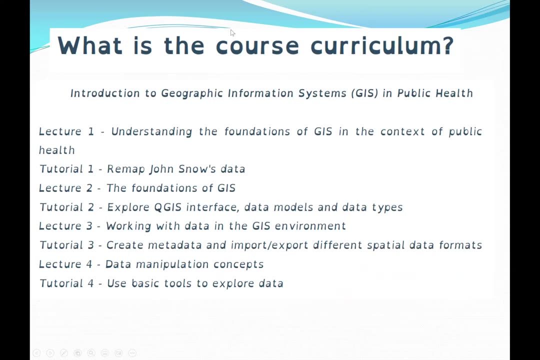 So we will get access to QGIS very quickly and either you are using Windows or Mac or Linus and QGIS is fine. You can run on the three major operating systems. So what is the course content? So the first thing: in lecture number one, we are going to 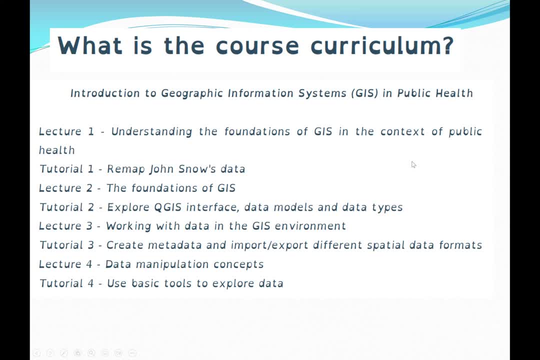 learn and also understand the foundations of GIS in the context of public health. Then we are going to do a lab work and this lab work, we are going to use the GIS to remap John Snow's data. We're also going to learn the foundations of GIS.